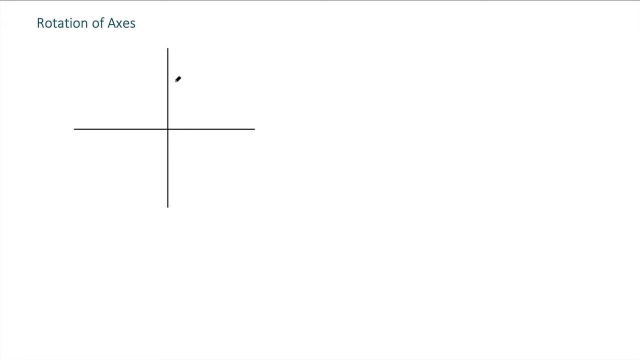 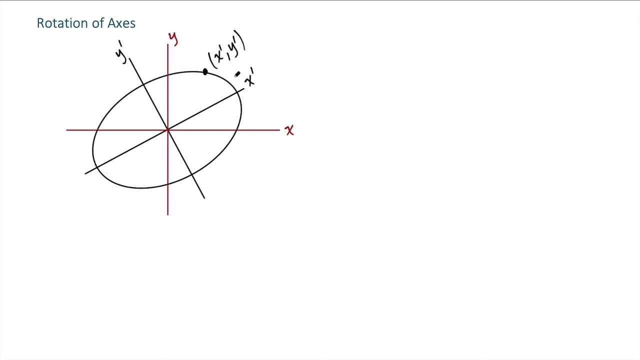 to rotate it. We're not supposed to rotate it, We're not supposed prime, y, prime, but we'll also call it just the point x, y, And the question is well, what is the relationship between those? So what we're going to do is actually just look at the 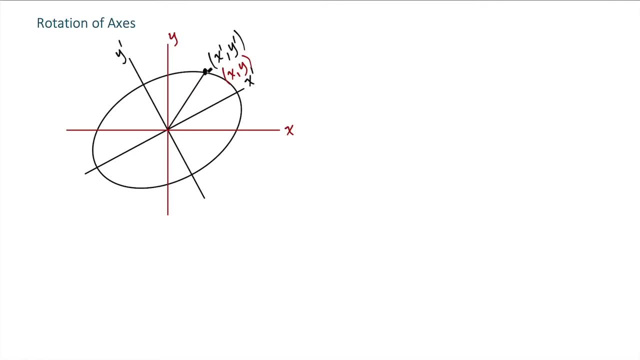 line from the origin and note that the origin is the same for both of these And we can look at a couple of different triangles. I'm going to first look at this connecting down to the x- y axis with a or to the x axis with a right triangle, And then I'm going to connect it to. 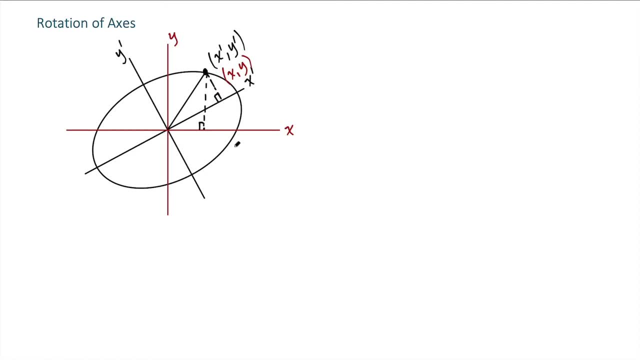 the x prime axis, okay, with another right angle. And now I can see: okay, there's some angles here to consider. Okay, this angle right here I'm going to call this angle theta, And this angle here I'm going to I'll call alpha, Okay, And then what we're going to do is we're going to 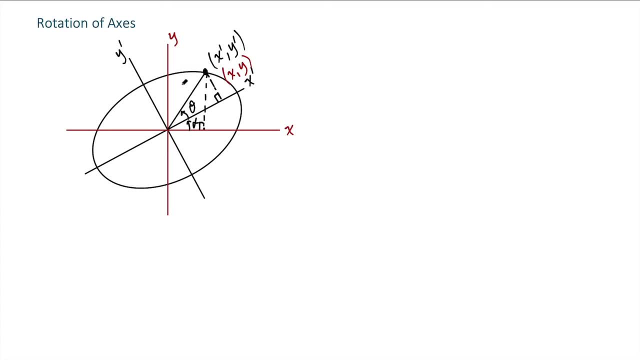 do is, oh, and also I'm going to label this distance right here as r, okay, the distance from the origin to our point. So alpha represents the angle of rotation and theta represents the angle that our point makes with the x prime axis. Now I can just write some relationships using 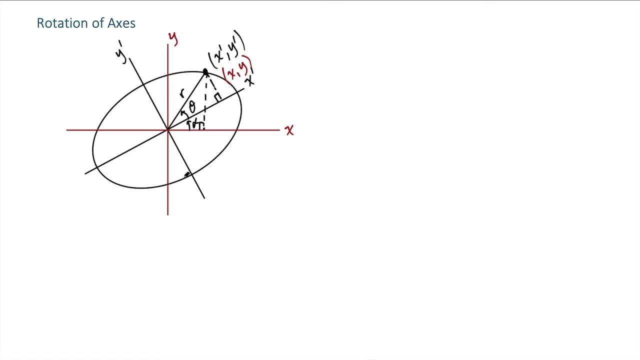 some trigonometric functions. I'll start in the x axis or the x? y system. Well, if I look at x- sorry, x right here- and this triangle which is has a theta plus alpha angle, I can do the cosine, the cosine of this. the sum of these two angles would be the x value. 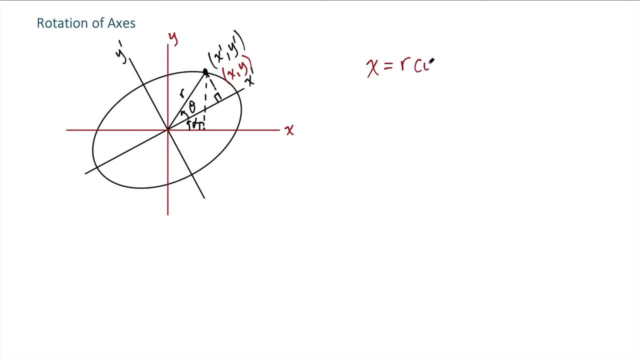 over r. In other words, x is equal to r times cosine of theta plus alpha. Okay, similarly, y equals r times sine of theta plus alpha. So that's looking at this larger triangle. here that comes down to the x axis. But we can also get a relationship between x prime and y prime. 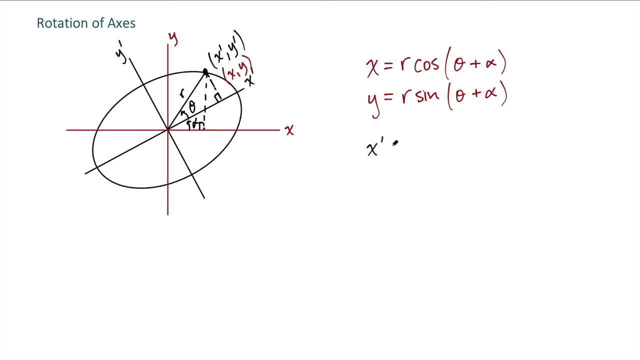 x prime is going to equal r cosine of theta cosine theta And y prime will be r sine theta. So I've got all these four different ways of locating this point: these two that are in the x- y system and these two that are in the x prime- y prime system. 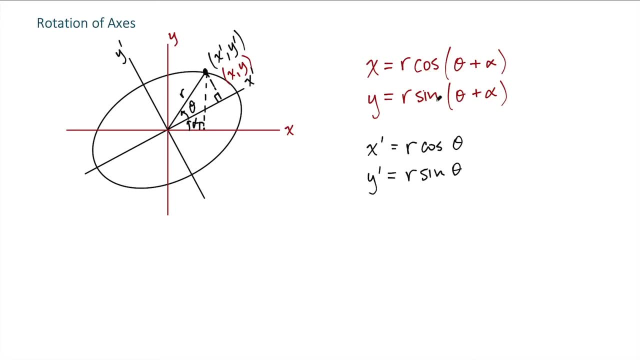 And now I can use the sum formulas for cosine and sine to rewrite the x and the y. So I'm going to go do that over here. So x is r times the cosine of theta plus alpha, is cosine theta, cosine alpha, and then minus, still r, r, and then sine sorry, sine theta, sine alpha. 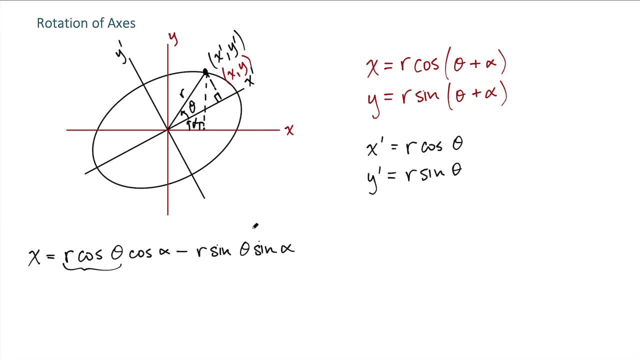 But I know that r cosine theta is x prime and I know that r sine theta is y prime. So then I get that this is x prime cosine theta minus y prime sine theta. And similarly I can look at y. Okay, y is r sine of theta. 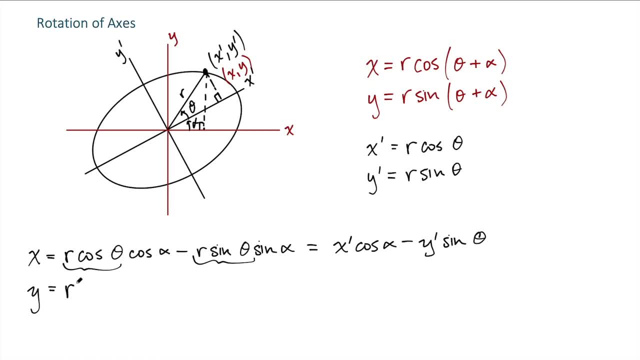 plus alpha. So again using my sum identity, there I get r? sine of theta, cosine of alpha, plus still r, and then cosine theta sine alpha, And then here r sine theta, that's y prime. so I have y prime cosine of alpha, and then plus r cosine theta is x prime sine of alpha. 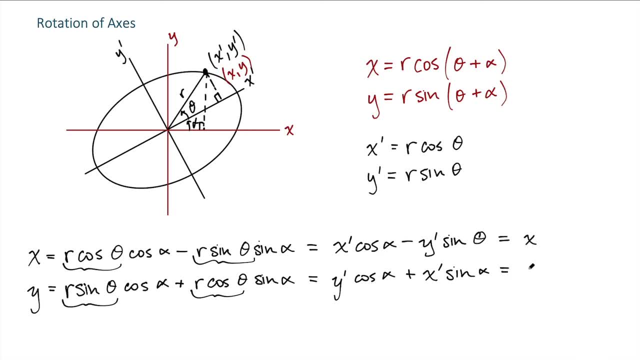 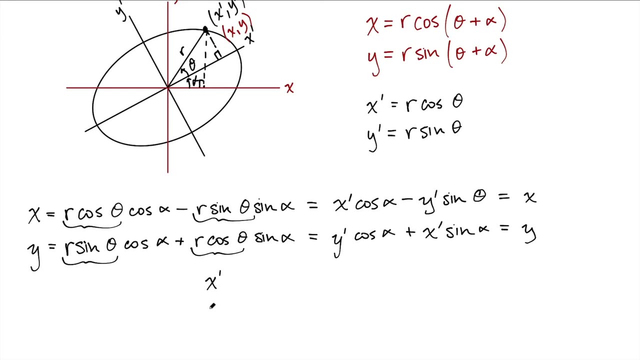 So these here. this is a relationship that exists between our x- y values and our x prime- y prime values. You can do a very similar process to get a relationship that takes us from x to x prime and y prime. I'll just go ahead and write the formulas that we get. 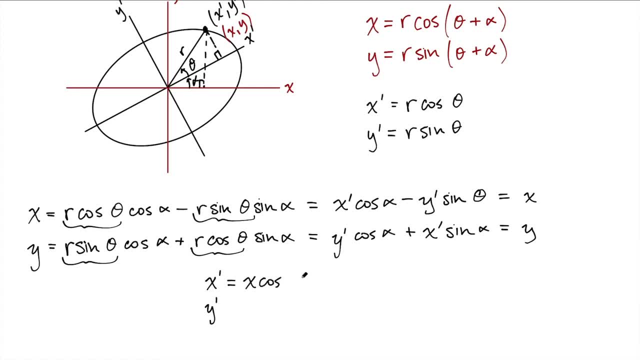 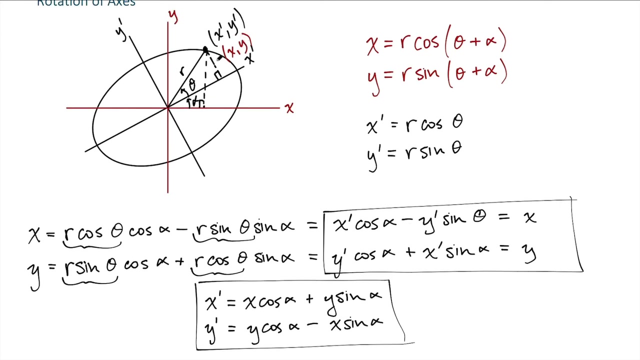 x prime is x cosine of alpha plus y sine of alpha, and y prime is y cosine of alpha minus x sine. So these are the formulas that relate the variables x prime, y prime and x and y. So anytime we want to rotate a conic we can find this angle of rotation alpha and we can put them in here or up here. 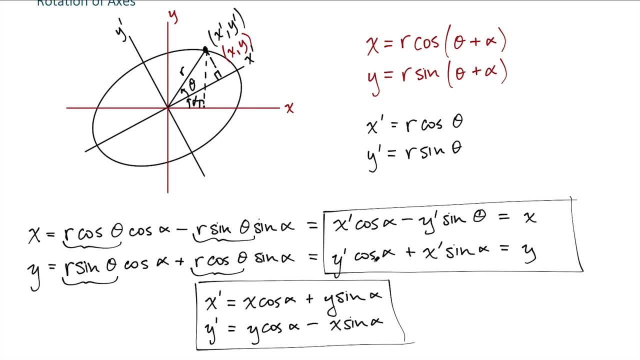 and then we can make replacements And then, in an equation for a conic to switch between an x- y system and an x prime- y prime system. Now, an important thing to know is that the standard equation of a conic, the most general that we can get, 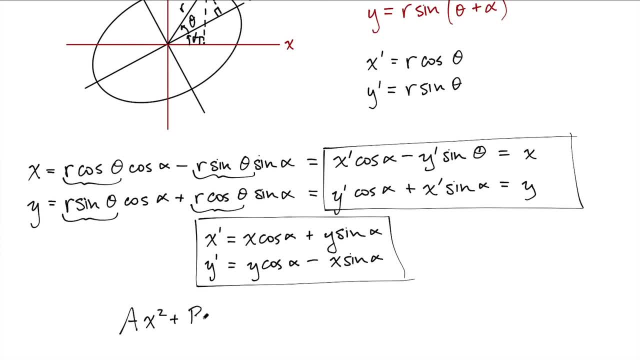 is going to look something like this: Ax squared plus bxy plus cy squared plus dx plus ey plus f equals zero. This is as general. This is as general as we can get. You'll note that we have this x- y term here. 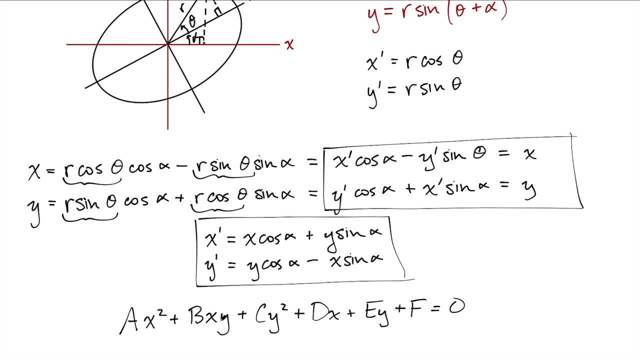 The presence of an x- y term- meaning if b is not zero- tells us that we have a rotated conic, And so if we're given a form that's like this, we can then take these expressions here: replace the x and the y with those, and this term will actually disappear.